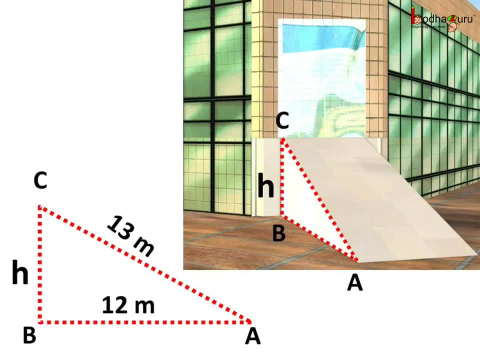 B is 12 meters, or you can say the base of the triangle is 12 meter, Height is h and it is the side BC. So according to the Pythagoras theorem, AC square is equal to BC square plus AB square, That is, the square of hypotenuse is equal to BC square plus AB square. 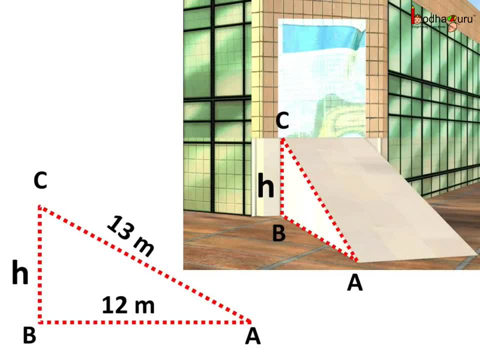 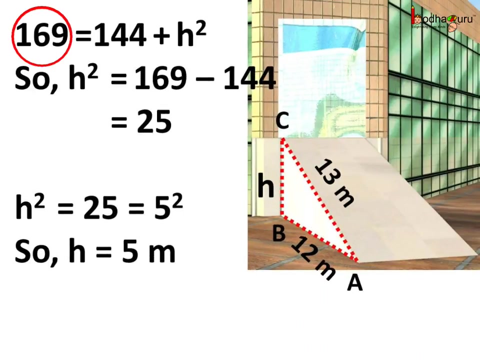 That is, the square of hypotenuse is equal to the sum of the squares of the base and the perpendicular. Thus we can say here: 13 square is equal to 12 square plus height square or the perpendicular square: 13 square means 169 and 12 square means 144.. 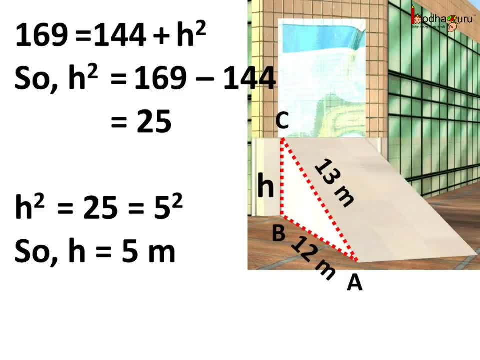 So h square is equal to 169 minus 144, which is equal to 25.. Now this means h square is equal to 25.. We know 25 means 5 square, So we can say h is equal to 5 meters and thus using the Pythagoras. 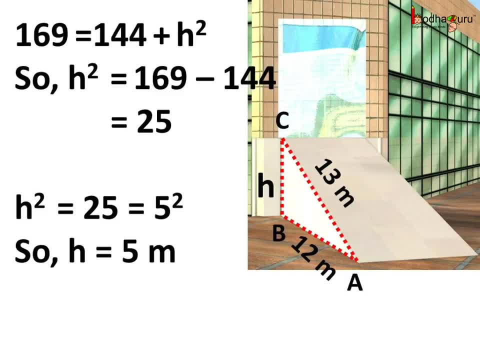 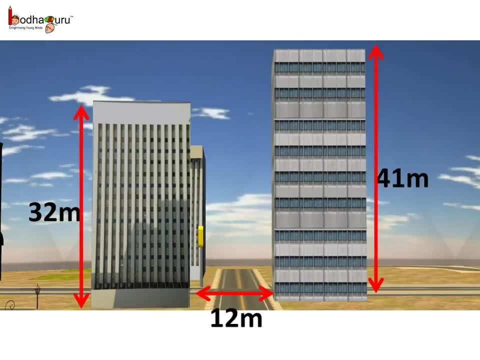 theorem, we found the height of this slanting plane. Let's take another example Here the distance between the two buildings is 12 meters. One building is 41 meters tall and the other building is 32 meter tall. Aman went to the roof of the shorter building and wondered what was the distance between the tops. 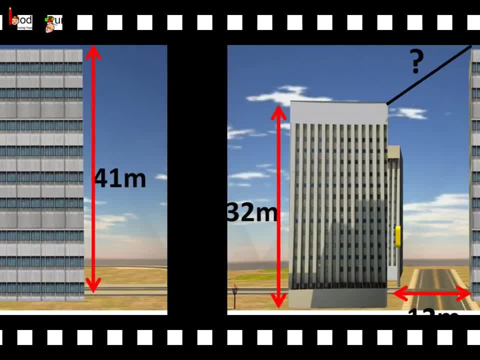 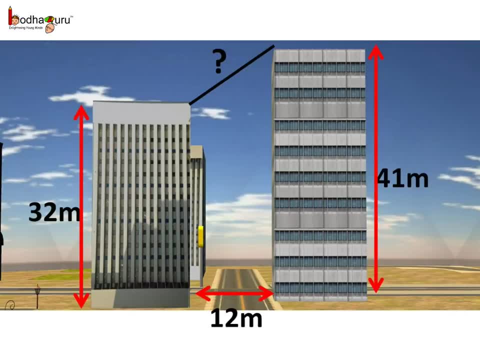 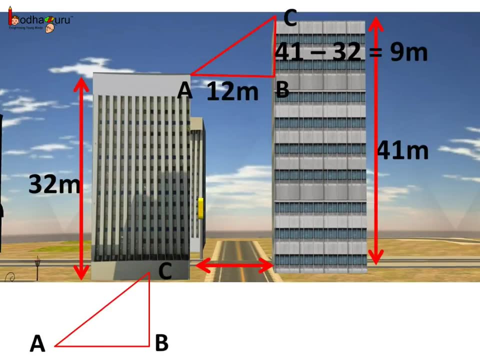 of the two buildings. Now, how to find distance between the tops of the two buildings? Well, here again we can use the Pythagoras theorem to solve this problem. Here we can draw right angle triangle, ABC. Look, the distance between the buildings is AB. 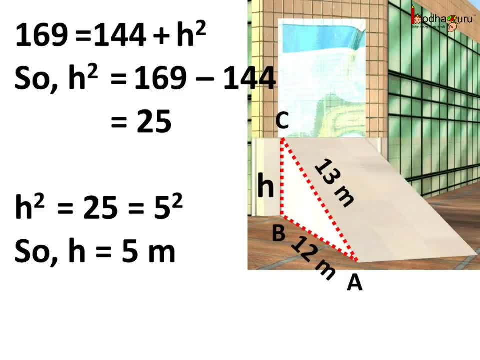 So h square is equal to 169 minus 144, which is equal to 25.. Now this means h square is equal to 25.. We know 25 means 5 square, So we can say h is equal to 5 meters and thus using the Pythagoras. 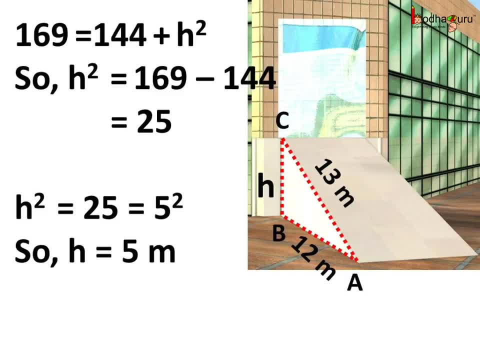 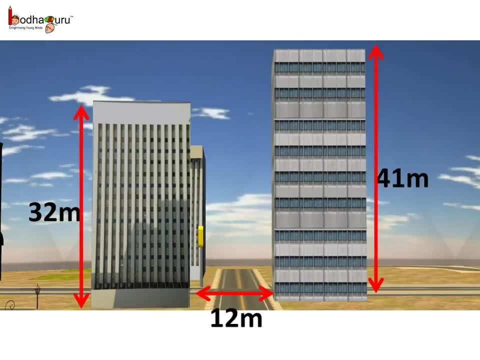 theorem, we found the height of this slanting plane. Let's take another example Here the distance between the two buildings is 12 meters. One building is 41 meters tall and the other building is 32 meter tall. Aman went to the roof of the shorter building and wondered what was the distance between the tops. 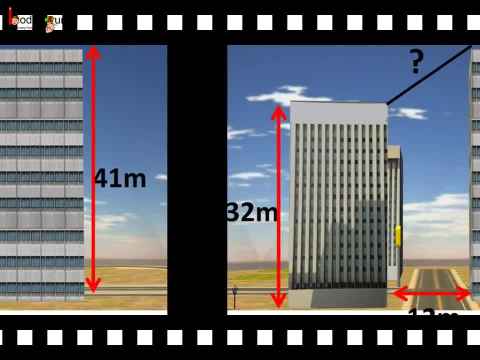 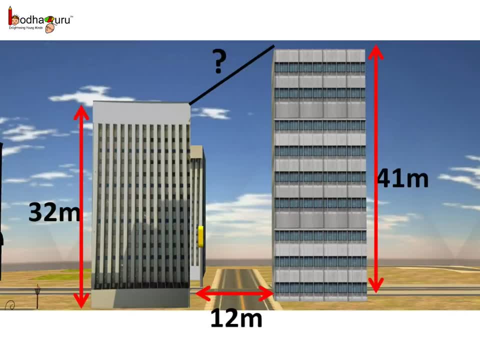 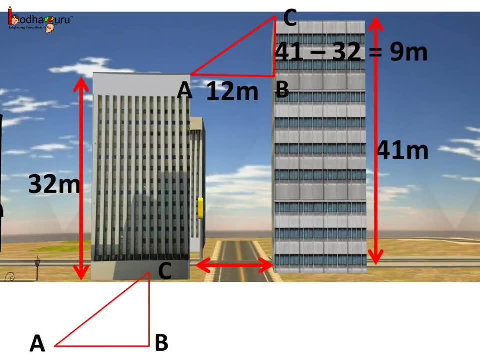 of the two buildings. Now, how to find this distance between the tops of the two buildings? Well, here again we can use the Pythagoras theorem to solve this problem. Here we can draw right angled triangle, ABC. Look, the distance between the buildings is AB. 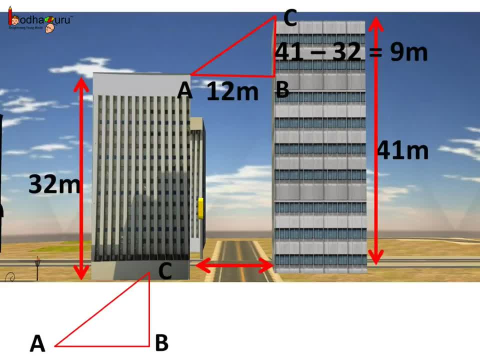 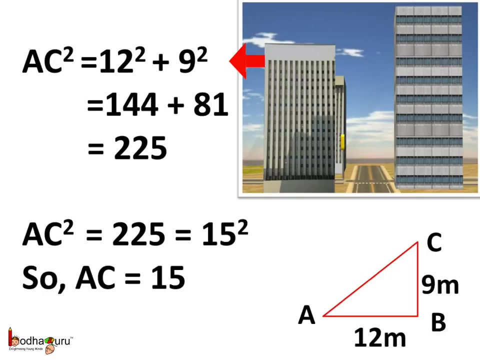 which is equal to 12, and the difference of the height is BC, and it is equal to 41 minus 32, which is equal to 9 meters. So we can say the distance between the tops of the two buildings is AC and, according to the Pythagoras theorem, AC square. 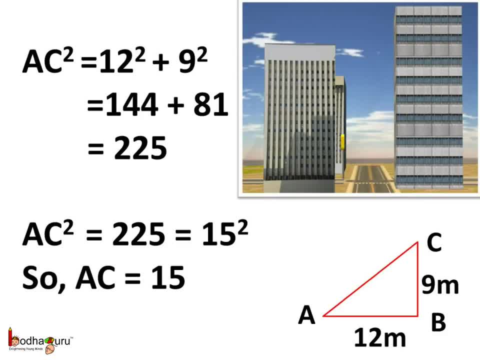 is equal to 12 square plus 9 square, which is square of the base plus square of the perpendicular. Hence AC square is equal to 225.. Now 225 is equal to 15 square, which means AC square is equal to 15 square, which means AC is 15.